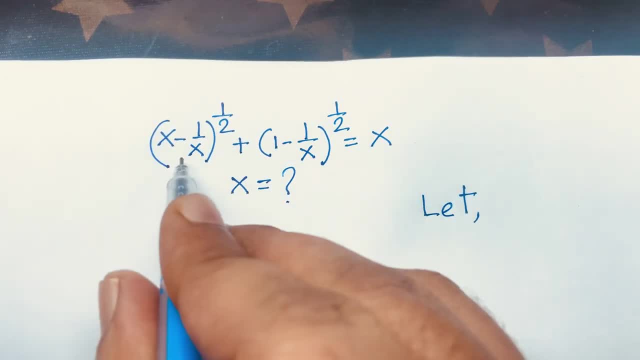 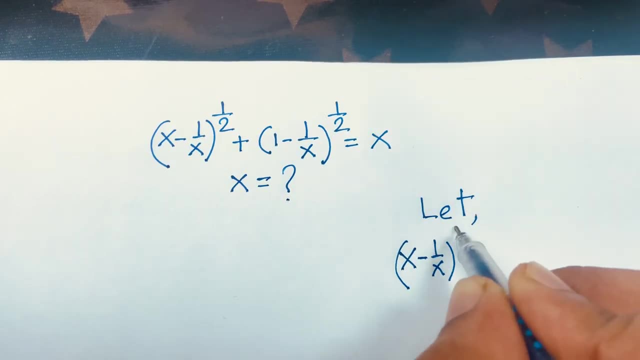 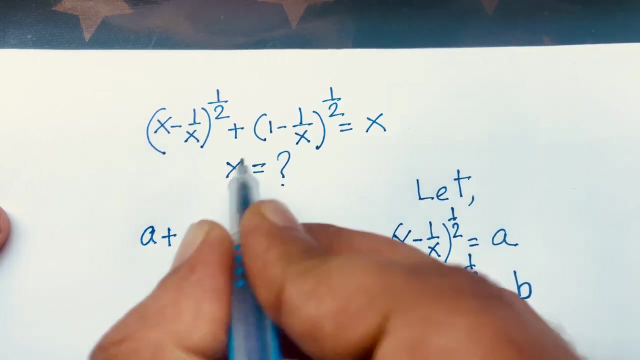 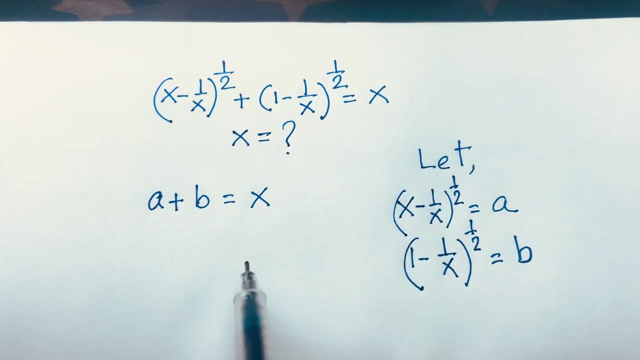 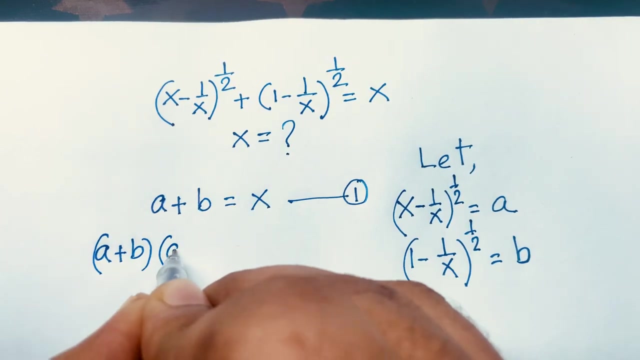 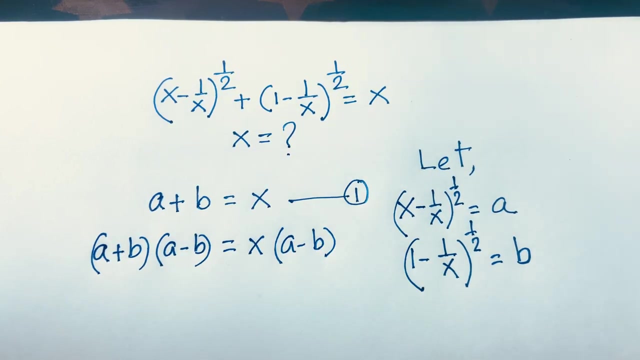 you want to solve this question, you need to find out what is the value of x in this math question. So, if you want to solve this question, you need to find out what is the value of x in this math question. So, if you want to solve this question, you need to find out what is the value of x in this math question. So, if you want to solve this question, you need to. 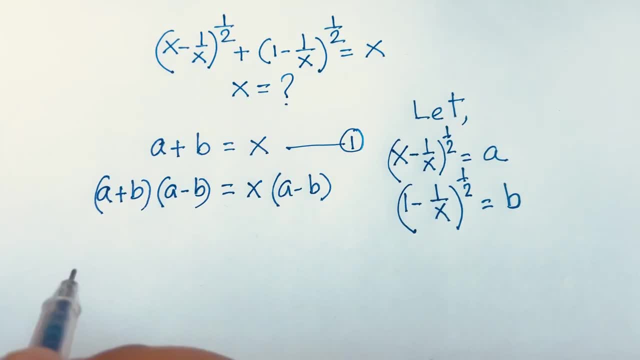 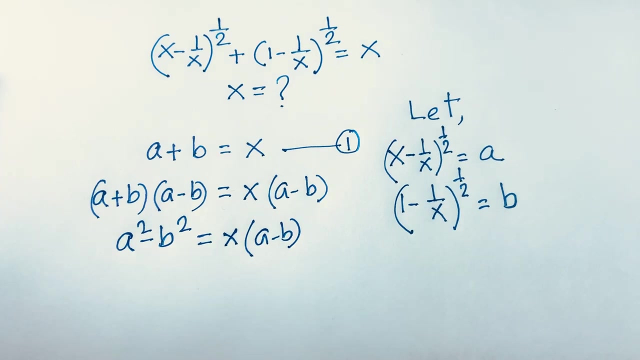 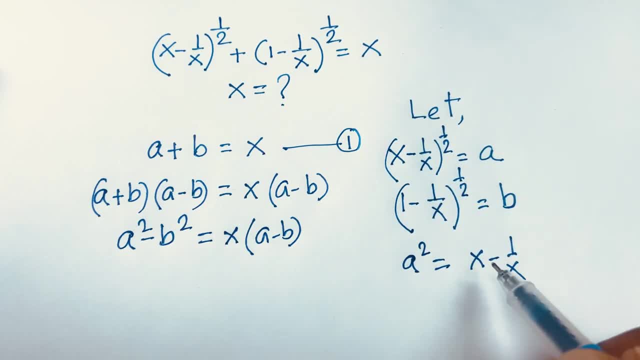 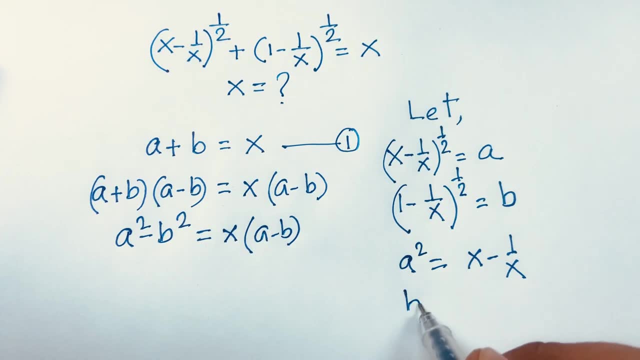 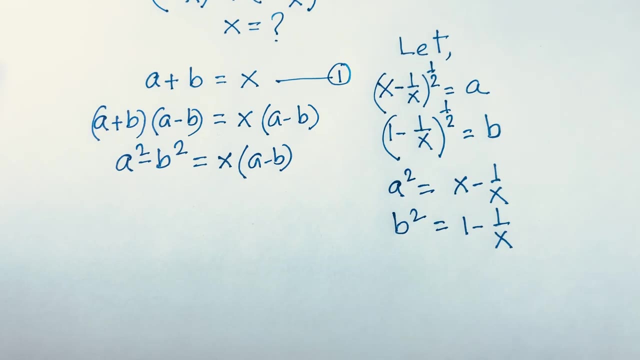 use both side, powers to, to, to cancel, we will find out. a square is equal to x minus 1 over x. and at this moment, if we use both side again too, so we'll find out, here is: b square is equal to 1 minus 1 over x. yes, but our need a square minus b square is equal to what? so at this moment, i can. 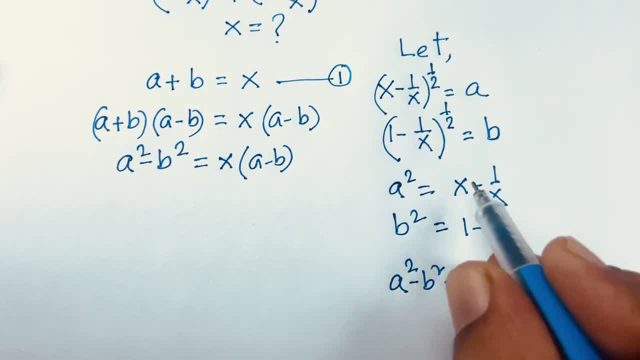 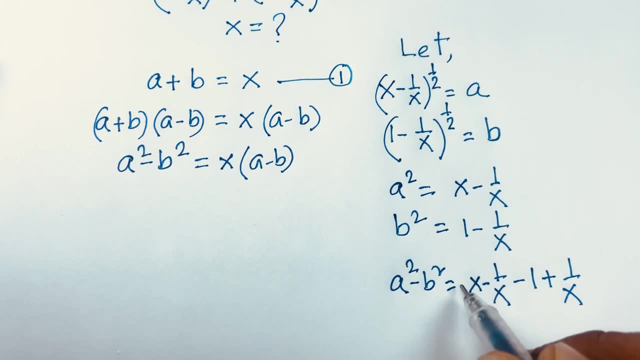 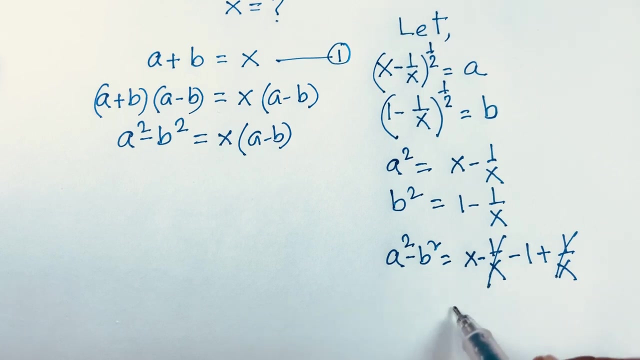 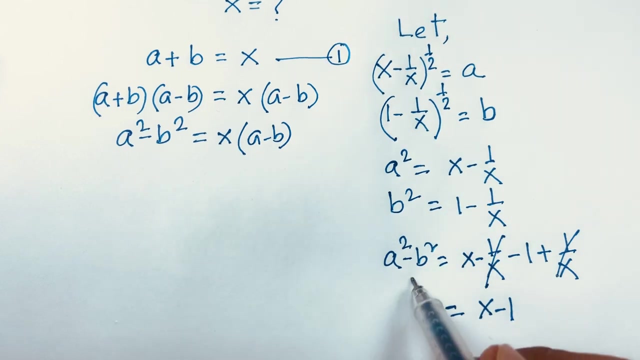 see easily a square minus b. square a is equal to x minus 1 over x minus b. square b is equal to 1 plus 1. over x minus minus, it will be plus. then i can see easily this, this cancel and we'll find out: here is x minus 1. yes, now, at this moment, i can see easily a square minus b square: it will be x minus. 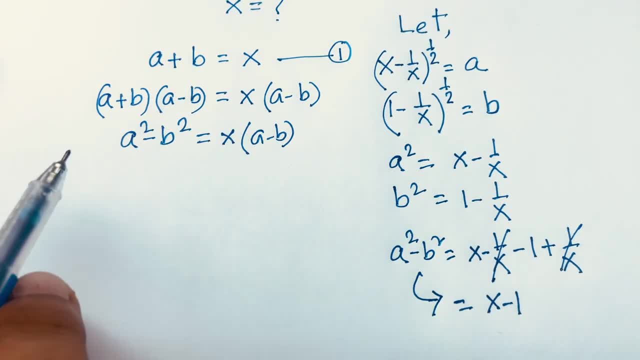 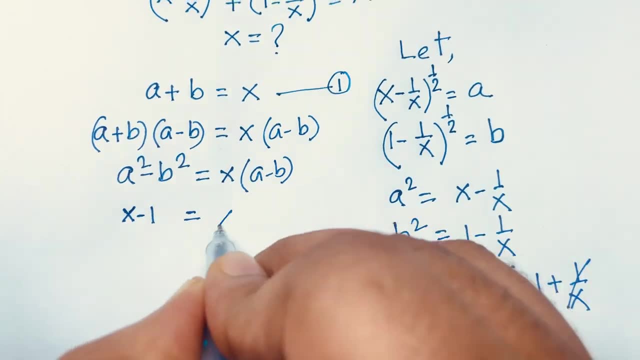 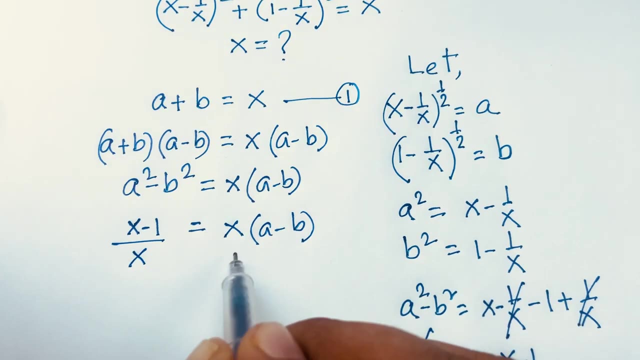 1. yes, so at this moment, if i put this value in this equation so i can see easily, it will be: x minus 1 is equal to x times a minus b. Now, at this moment, if I divide both sides by x: yes, so I can see. 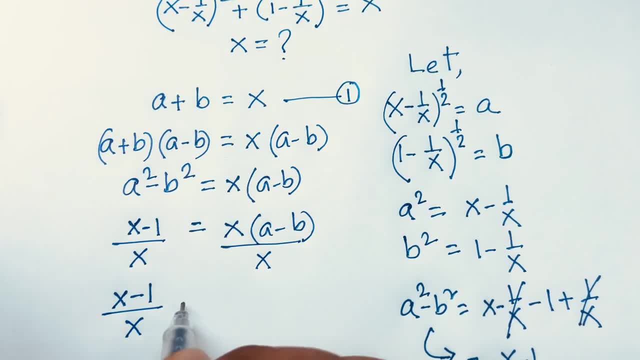 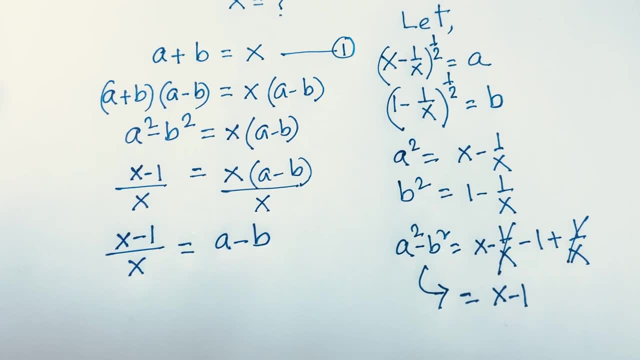 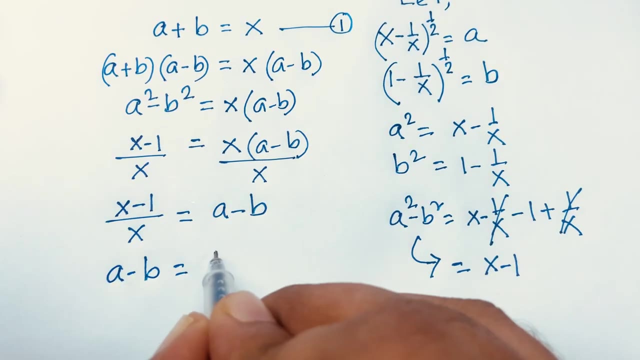 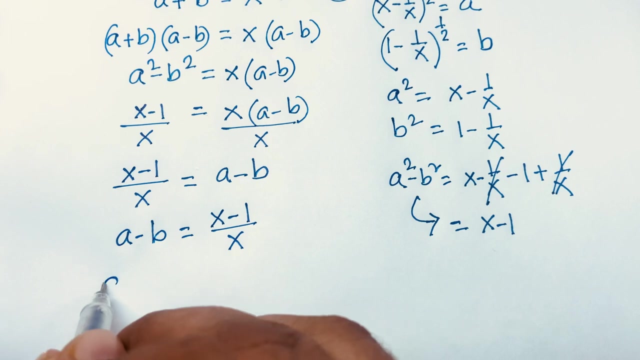 easily it will be: x minus 1 over x is equal to a minus b. Yes, x x cancel. we find out: here is a minus b. Now, at this moment, I can see easily: here is a minus b is equal to x minus 1 over x. Then this equation it will be: a minus b is equal to x divide. 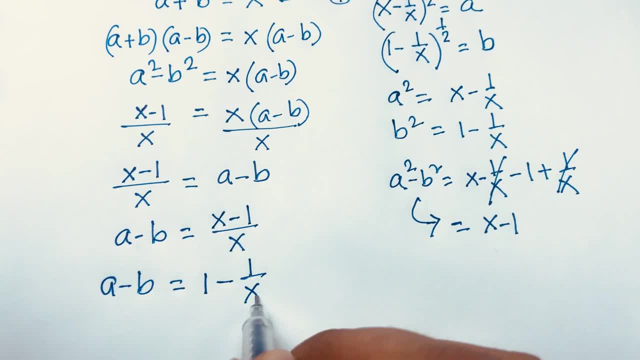 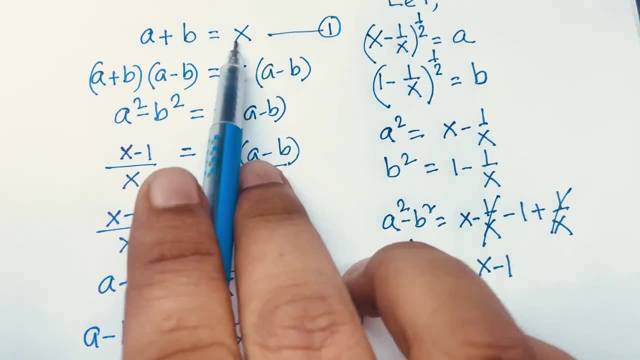 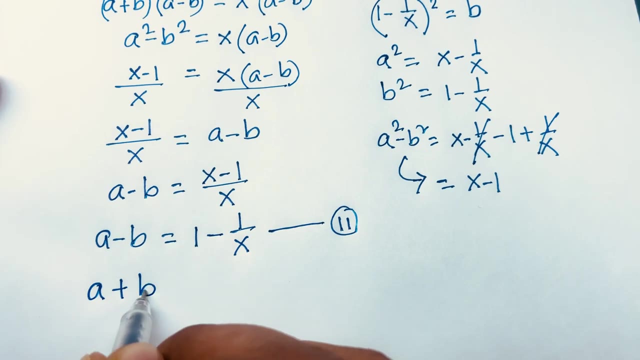 x, it will be 1 minus 1. divide x, it will be 1 over x. This is our second equation. Look, so our first equation is: a plus b is equal to x. yes, So our first equation is: a plus b is equal to x. 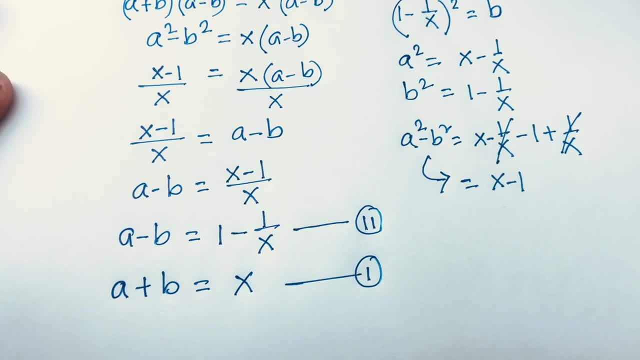 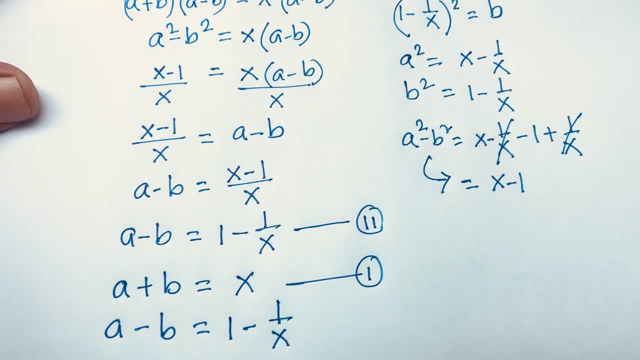 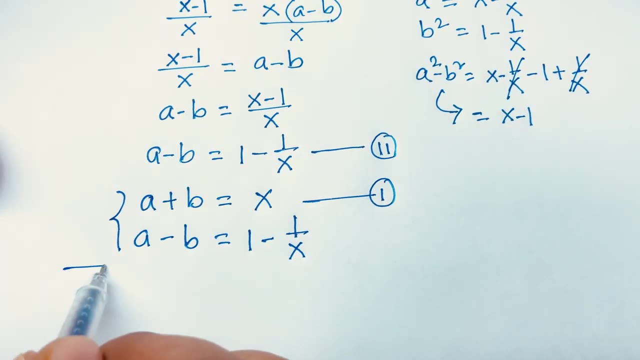 This is our first equation And we find out. our second equation is: a minus b is equal to 1 minus 1 over x. yes, Now, at this moment, if I add both equation- look this equation and this equation- this: 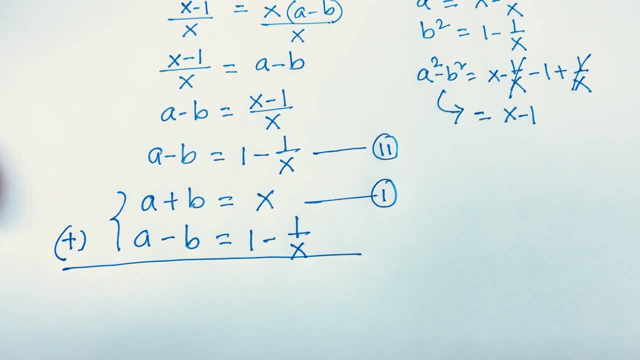 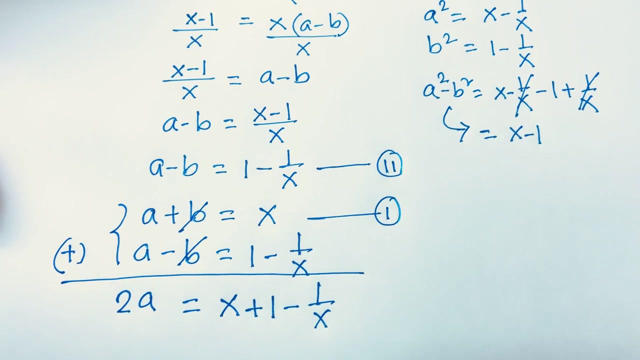 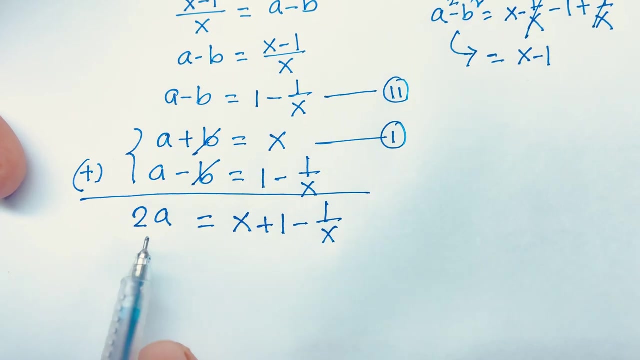 time I can say: I add yes, v, v, cancel. And we find out: here is a plus a, it will be 2a is equal to x. Now, at this moment, I can see easily it will be. look, I can see easily it will be. 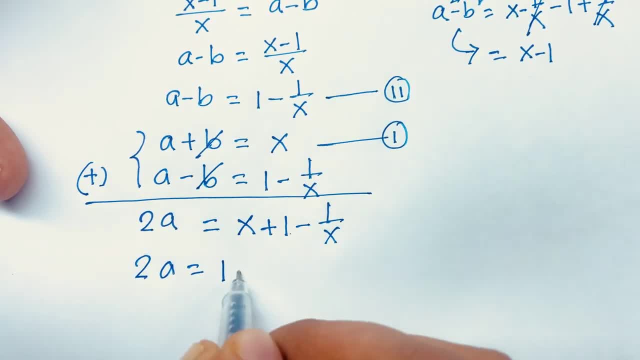 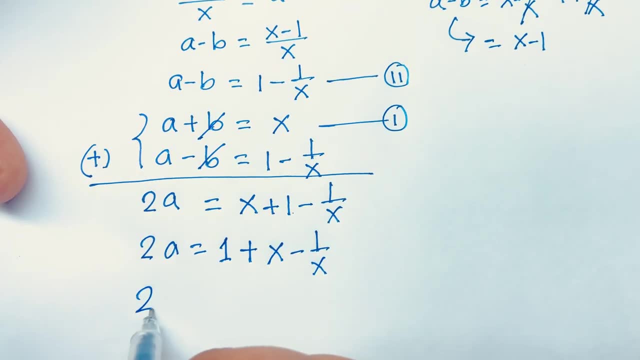 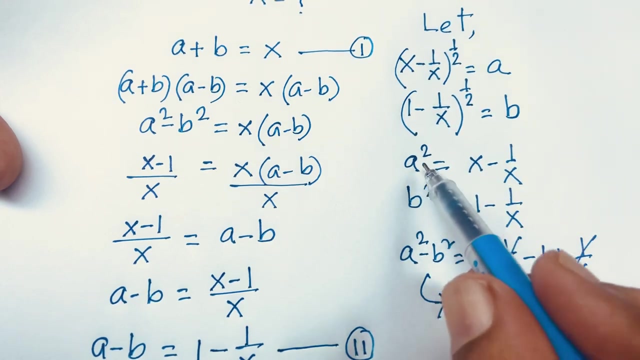 2a is equal to 1, yes, plus this, x minus 1 over x, this 1.. Now I can say 2a is equal to 1, plus remember that x minus 1 over x, It will be a square. 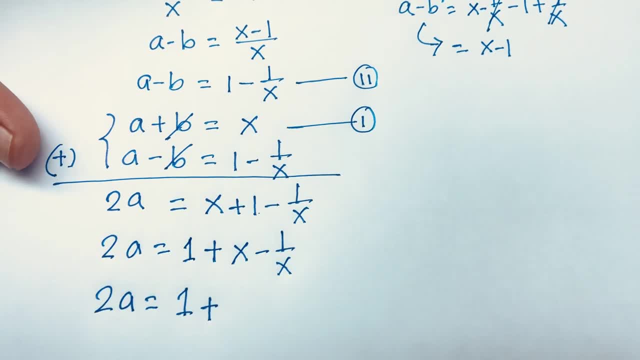 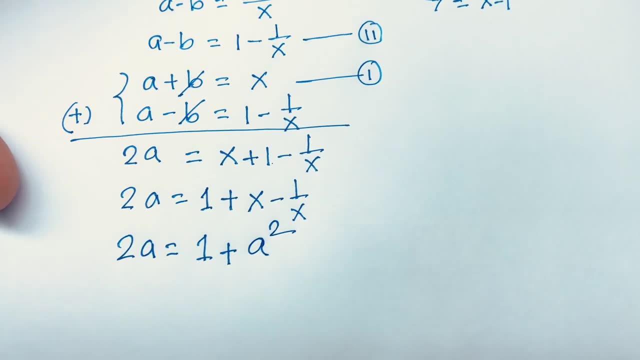 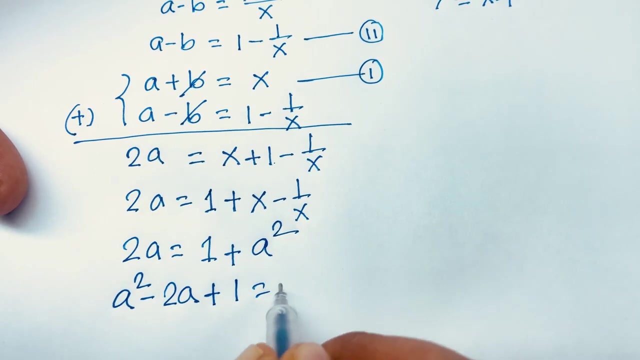 So if I put this below, in this equation we find out a interesting quadratic equation: x minus 1 by x it will be a square. Now, at this moment I can say this equation becomes a square: minus 2a plus 1 is equal. 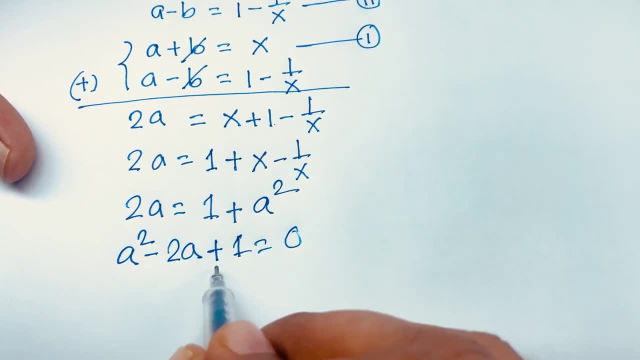 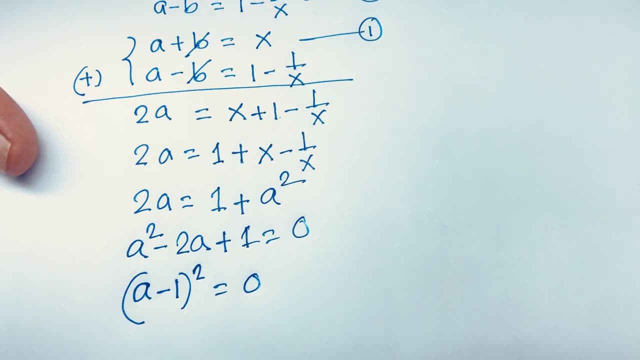 to 0. Then all of that, a square minus 2ab plus b square. according to this also, I can say it will be a minus 1, whole square is equal to 0.. Now then I can say easily: here is a minus 1 is equal to 0.. 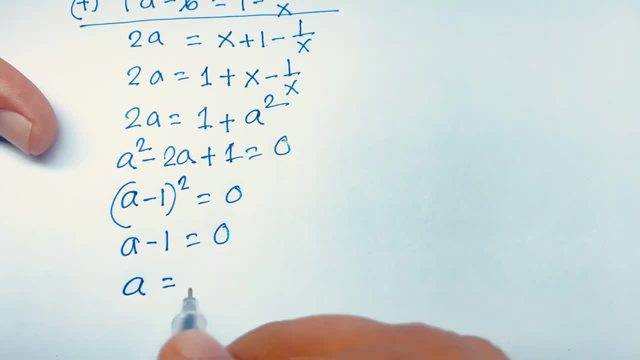 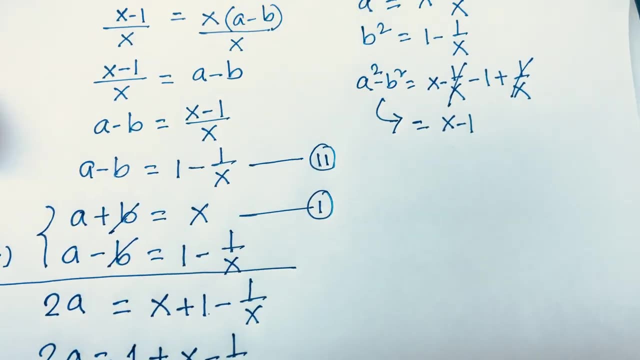 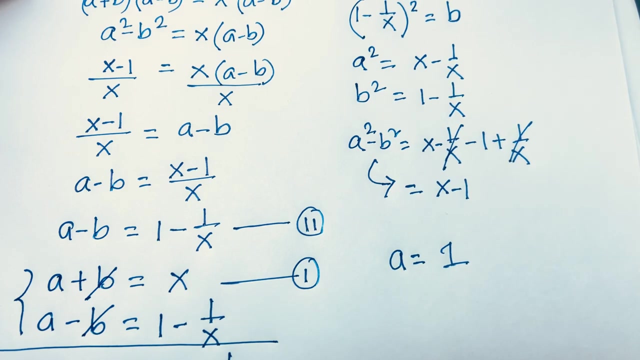 Then we find out a is equal to 1.. So finally, we find out a is equal to 1.. Okay, We find out in this question: a is equal to 1.. But our need x is equal to what? 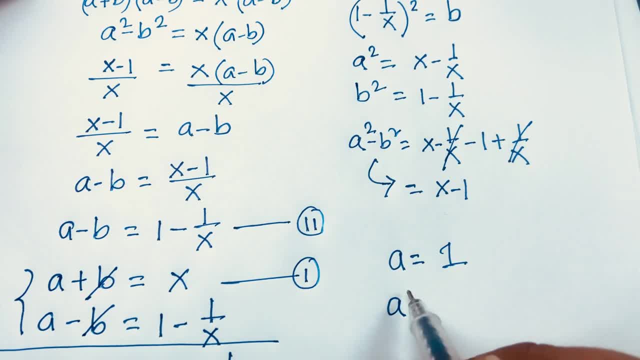 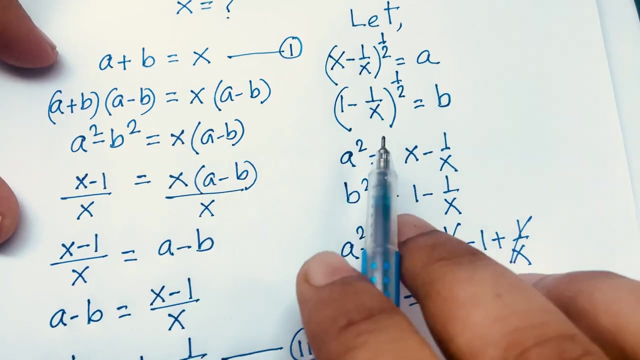 Yes. So I can say easily it will be: a square is equal to Look. remember that here is: a is equal to 1, but a square is equal to x minus 1 over x. So I can say easily: here is a look: a is equal to x minus 1 over x. whole to the. 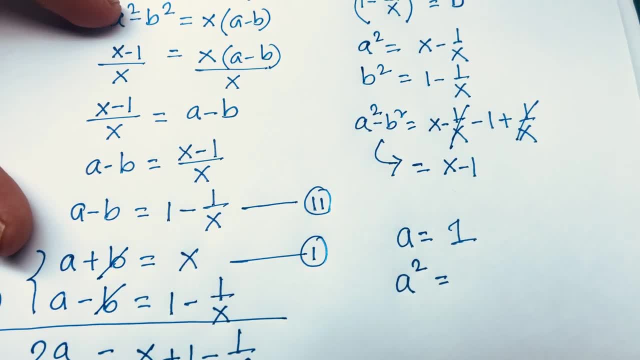 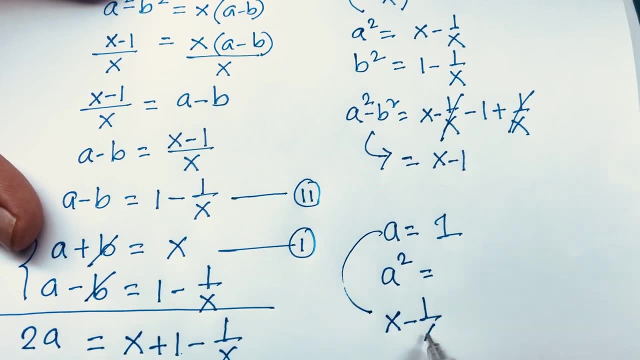 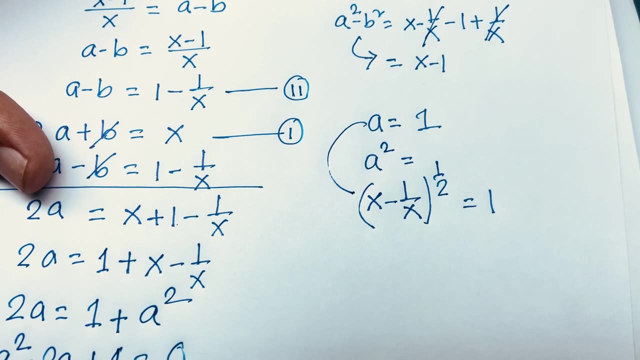 power half. So at this moment I can say easily: a look, it will be x minus 1 over x And a whole to the power half is equal to 1.. Yes, Now, at this moment, if I use both sides, power is 2.. 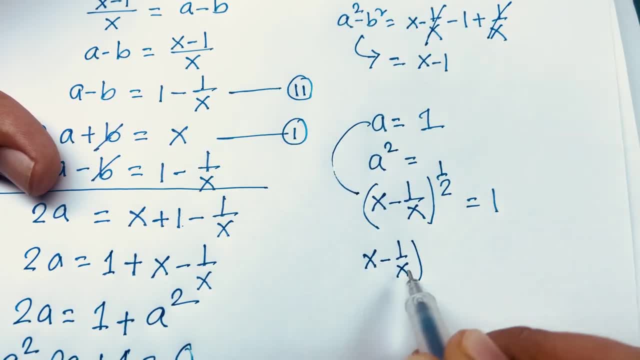 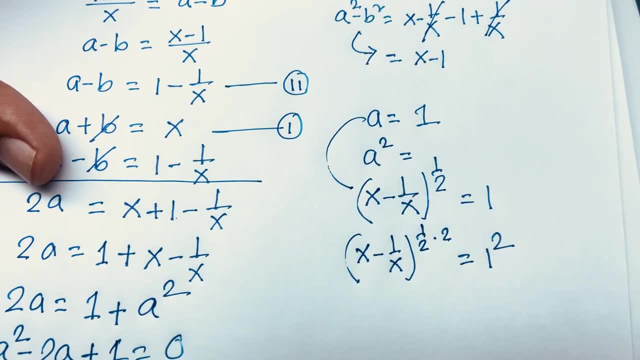 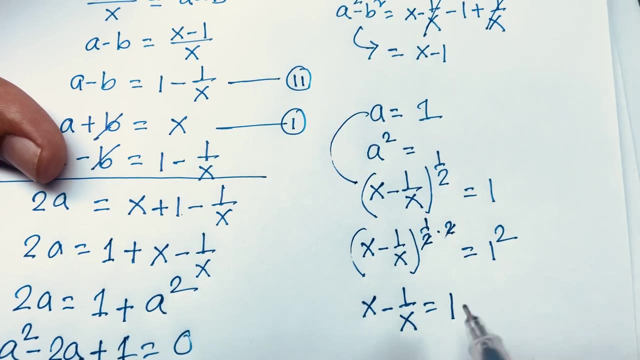 So we find out: x minus 1 over x and whole to the power, half times 2 is equal to 1 square. Now, at this moment, 2 to cancel we find out here is: x minus 1 over x is equal to 1.. 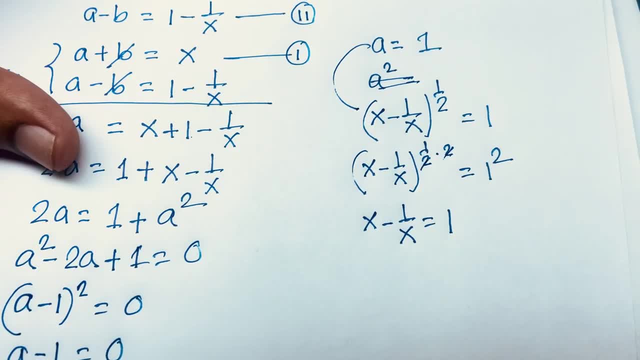 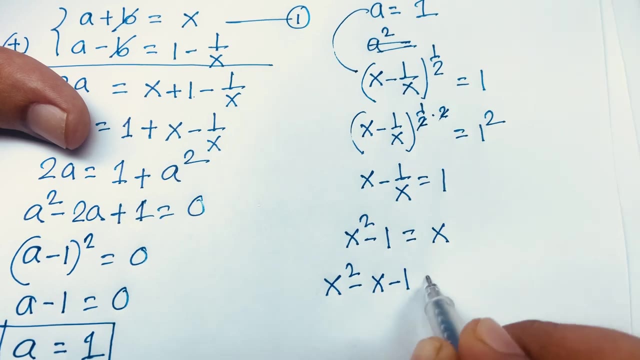 Now at this moment I can say easily: if I multiply every value by x, so I can say easily: it will be: x squared minus 1 is equal to x. Then we find out here: is x squared minus x minus 1 is equal to 0.. 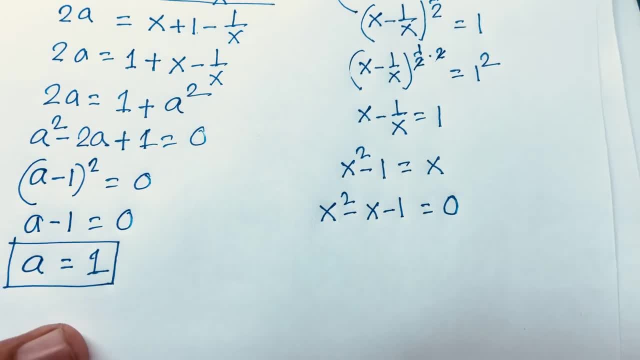 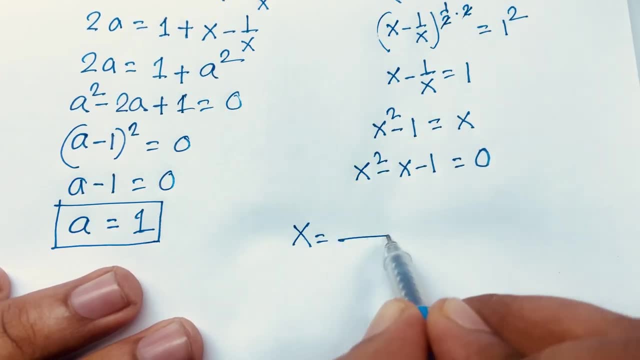 Yes, It is a nice quadratic equation. So at this moment, if I want to find out the value of x in this question so I can say easily: here is x is equal. Here is x is equal to minus b, Here is b is minus 1.. 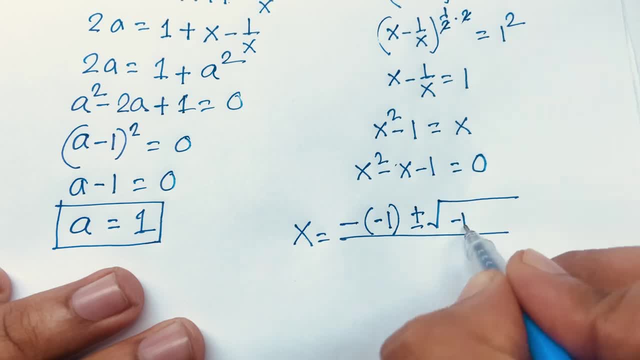 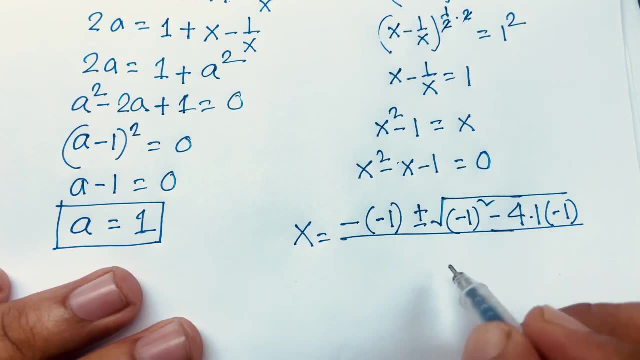 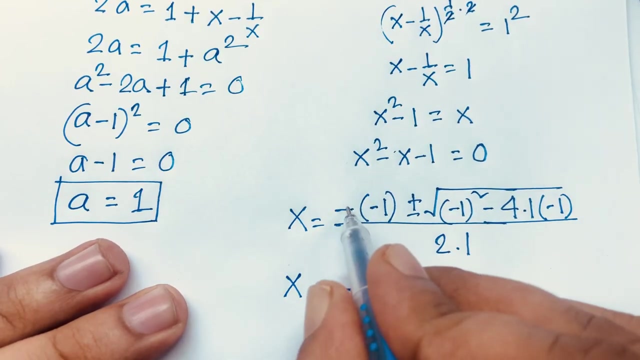 And plus minus square root b. square b is minus 1, whole square minus 4ac is 1 and c is minus 1. over 2a is 1.. Now at this moment I can say easily: x is equal to minus minus it will be positive 1..